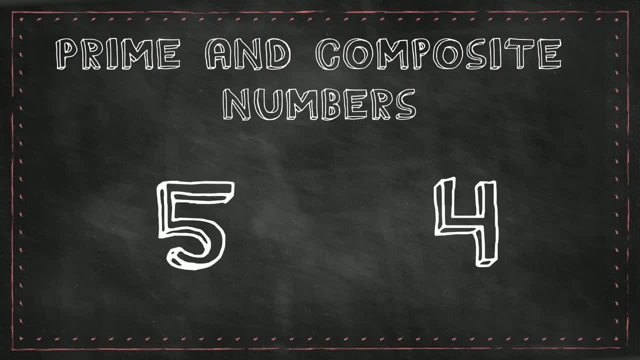 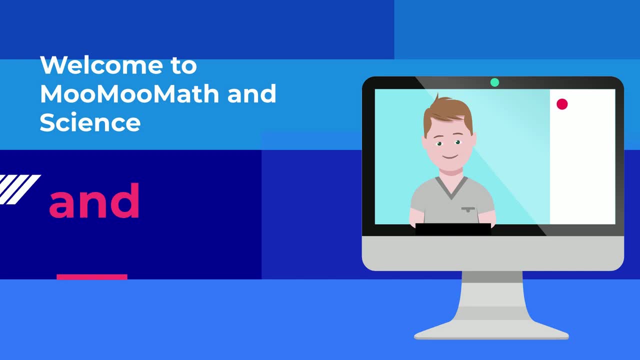 If you take a look at the numbers 5 and 4,, which number is prime and which number is composite? Welcome to MooMooMath and Science and the difference between prime and composite numbers. Let's begin by looking at the rules for prime. 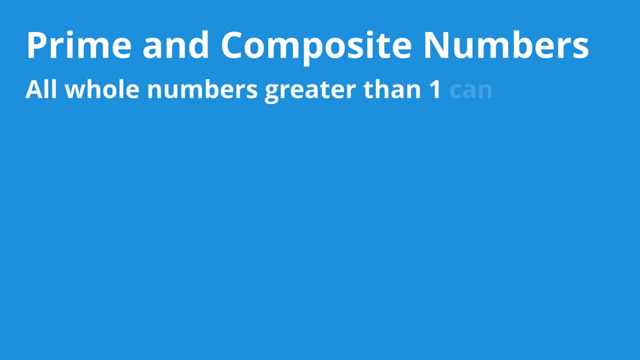 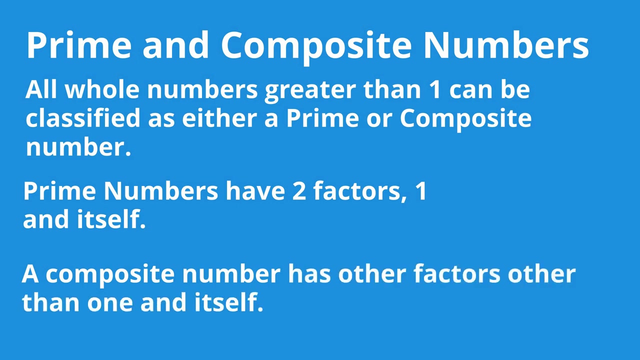 and composite numbers. All whole numbers greater than 1 can be classified as either prime or composite numbers. Prime numbers only have two factors: 1 and itself. A composite number has other factors other than 1 and itself. So let's take a look at some examples. 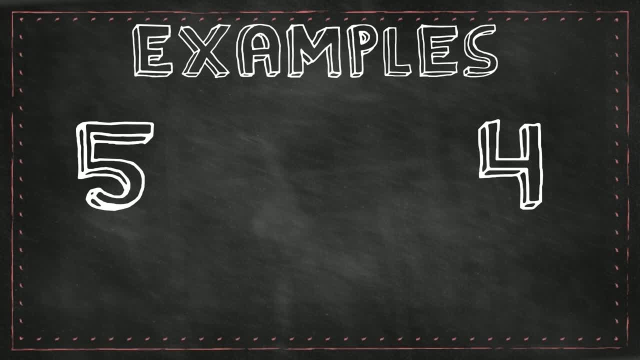 Let's look at 4 and 5.. 4 is divisible by 1, and 4 is also divisible by 2.. So 4 is a composite number, 5 is divisible by 1, but it is odd, so it is not divisible by 2 or any other number. 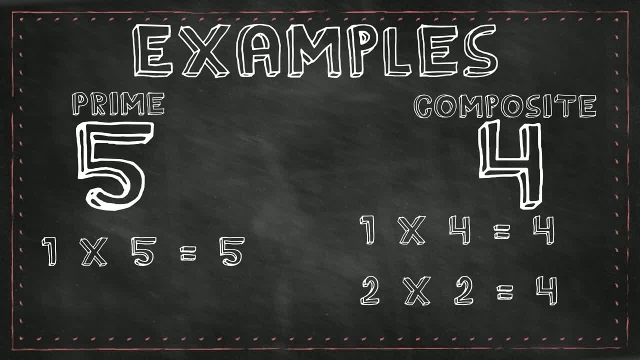 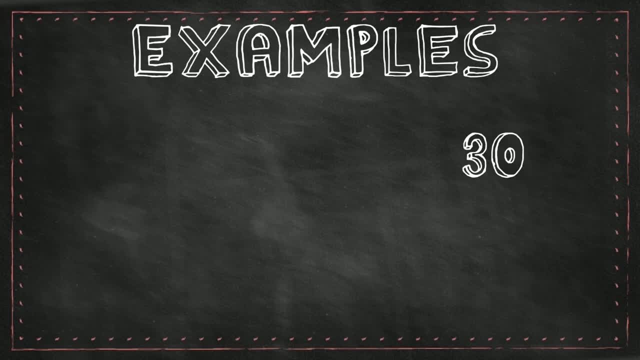 So 5 is a prime number. So let's look at a couple numbers that are a little bit larger. Let's look at 30 and 31.. 30 is divisible by 1. It is even so. this means that it is also divisible by 2. So you already know that it is a composite number. 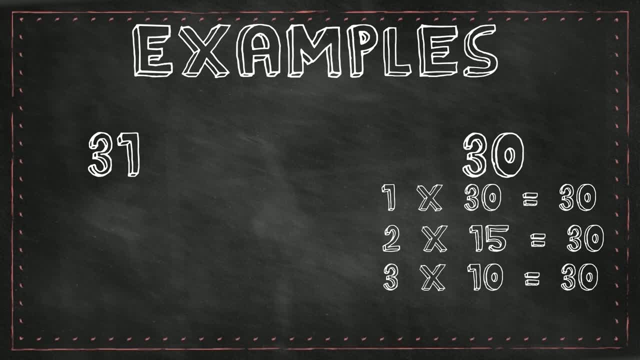 but it is also divisible by 3 and 5.. So again, 30 is a composite number, So 5 is a prime number. 31 is divisible by 1.. It is not divisible by 2 because it is odd or 3 or any other number. 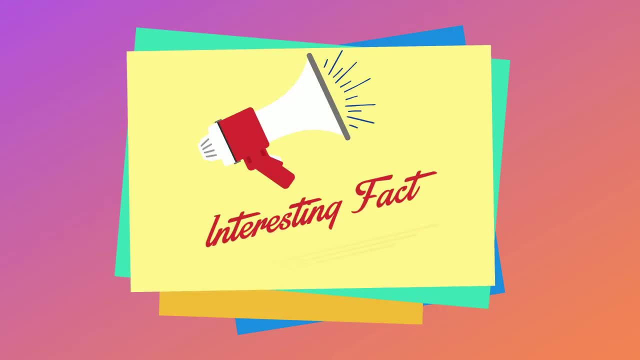 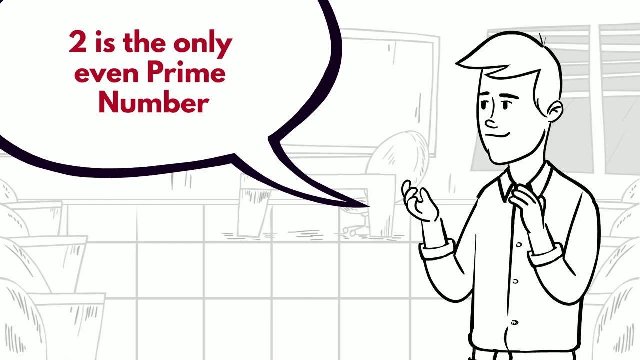 So it is going to be a prime number. Okay, interesting fact: 2 is the only even prime number. Any other number that is even will be a composite number because it is divisible by 2.. So, in summary, prime numbers are only divisible by 2 numbers, So it is divisible. 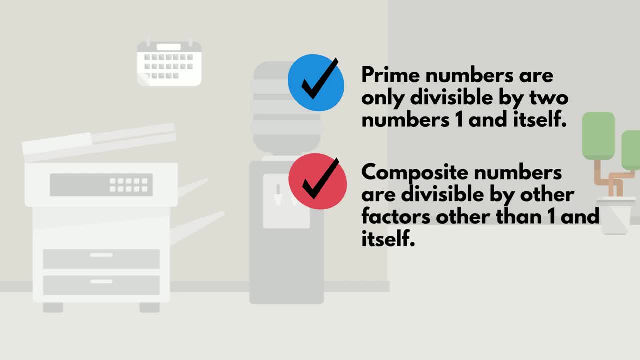 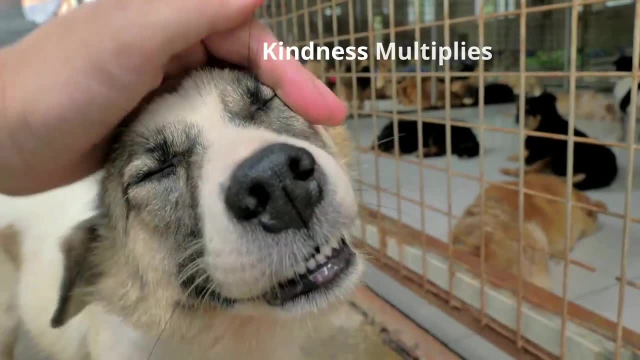 by 1 and itself. Composite numbers are divisible by other factors other than 1 and itself. Thanks for watching and remember: kindness multiplies kindness. Be kind to someone today.